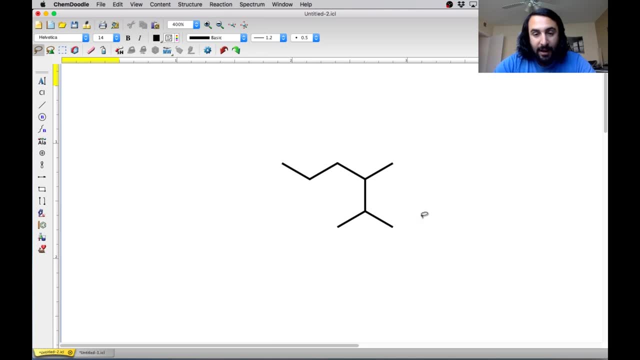 2,, 3,, 4,, 5,, 6.. And then we've got methyls on 2 and 3.. So, just to make sure that we're right, let's go ahead and add that name. Okay, So we've got 2, 3-dimethylhexane, like we said. So here's. 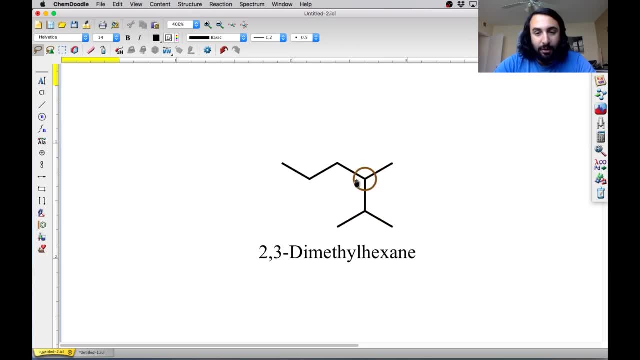 1, and then 2 has a methyl, 3 has a methylhexane, So we've got 2, 3-dimethylhexane, So we've got methyl 4, 5, 6.. That's correct. Just to show you a feature here. this is fun. You can alter it. 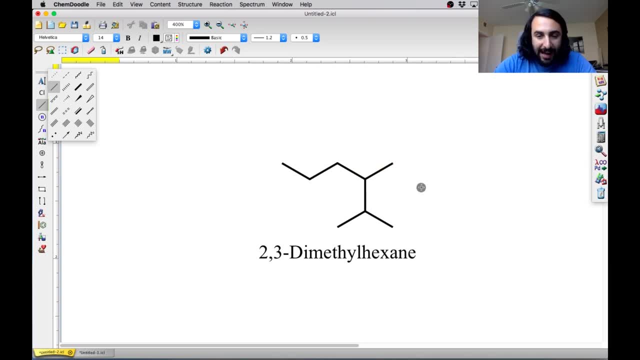 as you go. So how many carbons do we have to attach here to make this side to side, this left to right chain, the longest chain? Well, okay, So what have we done here? Now? it's still this right. It's still 1, 2-methyl, or, sorry, 2 on the methyl 3, we have an ethyl 4,, 5,, 6.. So 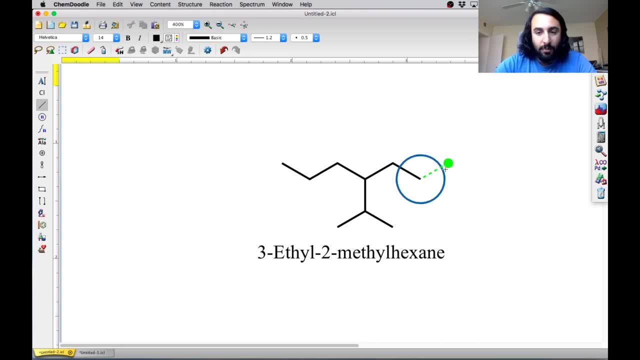 that's still keeping the same parent chain that we had before, If we add one more. finally, we've got this. This is now the parent chain, and this has become an isopropyl group instead of part of the main chain. So that's that one. That was just a quick warm-up, because now I want to get to the 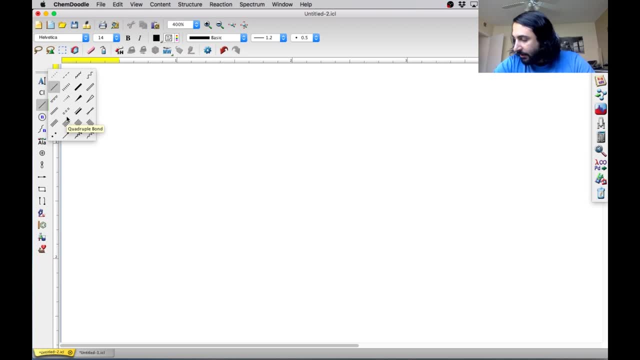 polycyclic stuff. We've already done that kind of stuff, So let's go over some new things that we have not discussed the nomenclature for. So let's take this, let's put this over here, And this is called naphthalene. Okay, So when you 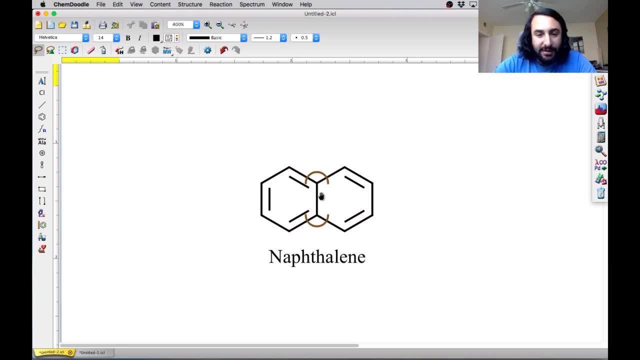 have two benzene rings like this. they're fused at these two carbons. This is now called naphthalene. So what happens when we start attaching things here? Well, okay, So, let's put a methyl over here, So 1-methyl naphthalene, Okay So. but let's look at something. This is: 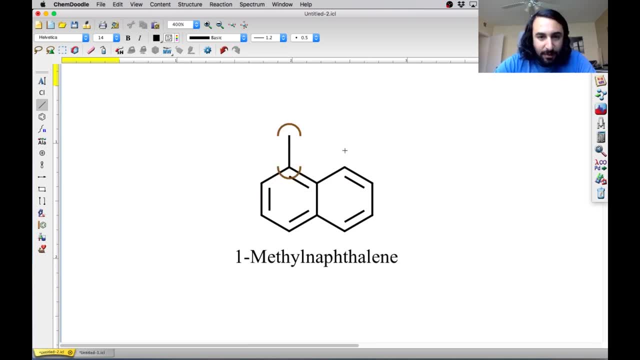 a. this is why this is a cool feature. We can- we can- see what happens if we do different stuff, Instead of having to draw a bunch of structures for you. we can do this very quickly. So we see that this is also 1-methyl. What if I put it over here? This is also 1-methyl again. And lastly, 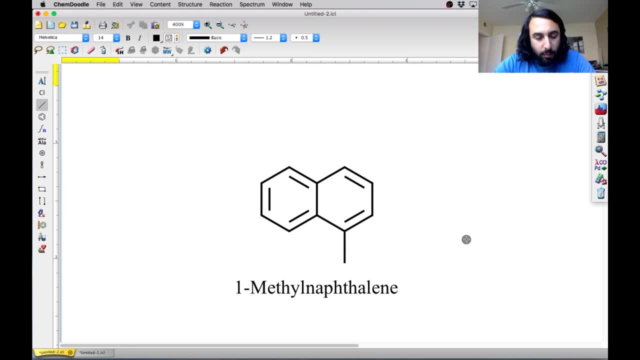 this is also 1-methyl. And so what? what do we? what does that tell us? Well, these are all identical positions at first, because we can rotate that molecule right. We can rotate it any way we want, We get the same thing. So that's why all those positions are identical. But let's say we put the 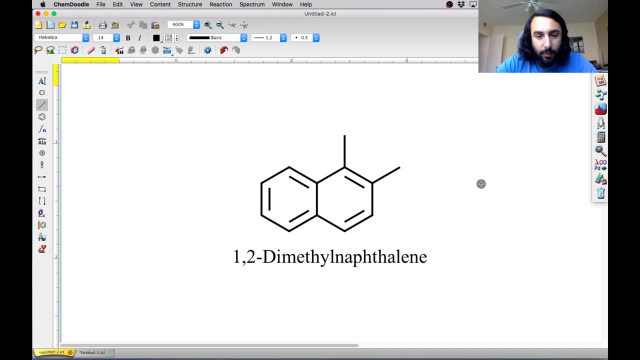 one there. Where can we go? All right? Well, what is this? So we've got 1,, 2.. So clearly we're going to be numbering in this way. This looks like position 3.. This will be position 4.. Now what? 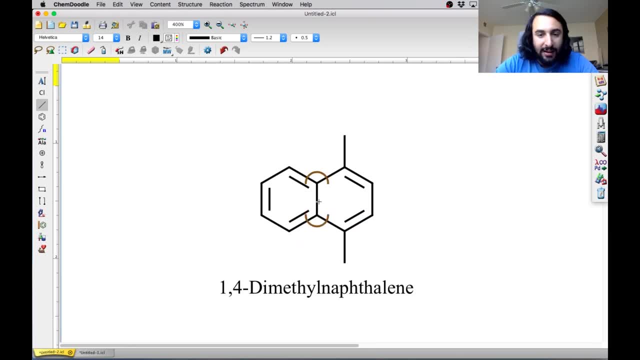 about this. This cannot accommodate a bond, So we're actually not going to count these two carbons in the numbering scheme, So this will be position 5.. This would be 1, 5-dimethyl. This would be 1, 6-dimethyl. This would be 1, 7-dimethyl, And then, lastly, this would be 1,. 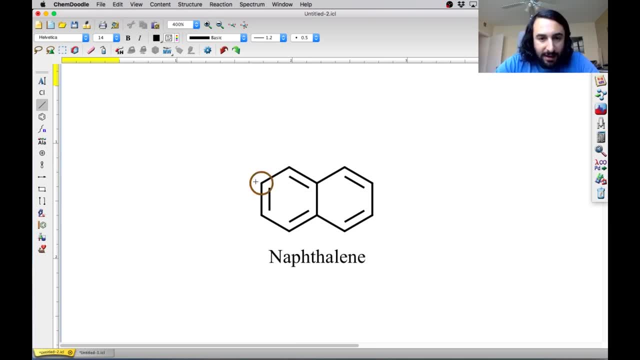 8-dimethyl. Now what if we start with something else? Let's put it over here. Now we've got 2-methyl, So that's counting this as carbon 1.. So this has changed what we count as carbon 1.. So let's take that and then let's add another one. Let's go over here, But now. 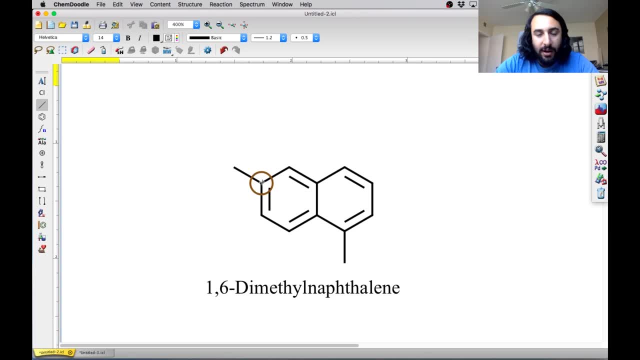 look at what happened. We did not keep this as carbon 1.. We did not keep this as carbon 1.. We did not keep this as carbon 2 and this as carbon 1.. Remember that we're going to number it so as to give the lowest set of locants to the substituents. So before this was carbon 1 and 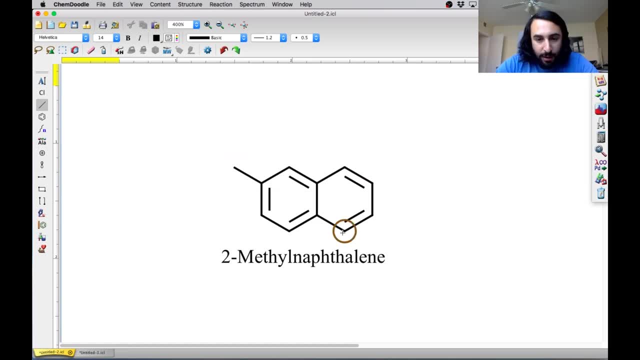 this was carbon 2 and we had 2-methyl naphthalene, But if we put it over here, it's automatically going to count this carbon as carbon 1.. Remember that any of these four could have been carbon 1.. 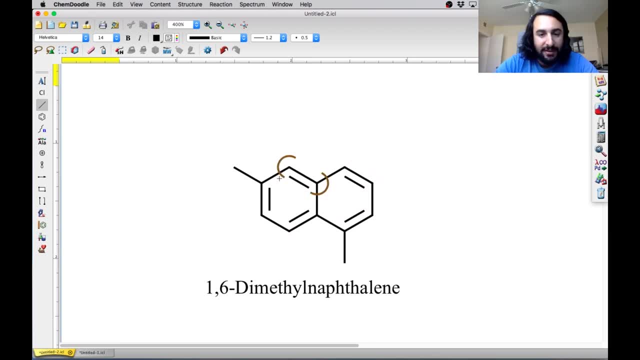 And if it does this, now we've got 1,, 2,, 3,, 4,, 5, 6.. 1, 6 is lower than if we went 2,, 3,, 4, 5.. So that's going to be a better numbering system for that And we can just draw. 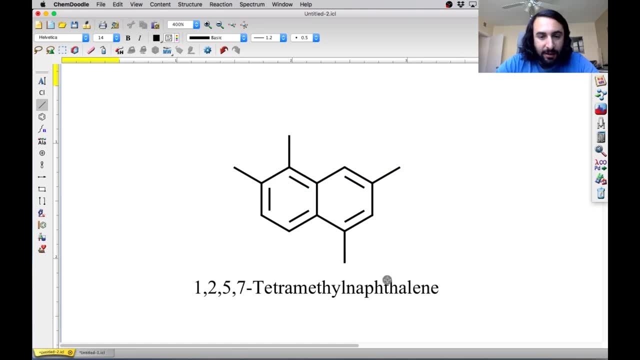 methyls everywhere and see what ends up happening. We can just look at the name So clearly this is 1,, 2,, 3,, 4,, 5, 6, 7 tetramethyl instead of 1,, 2,, 3,, 4,, 5, 6.. So we always want the lowest set. 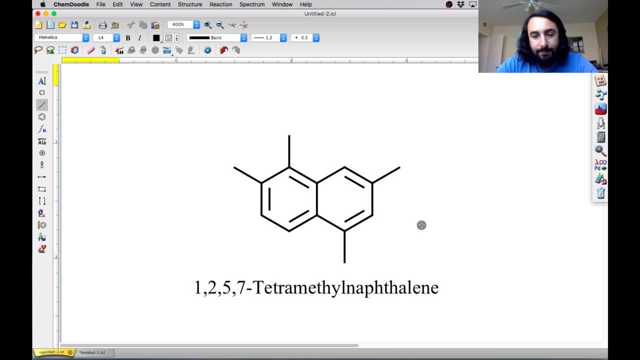 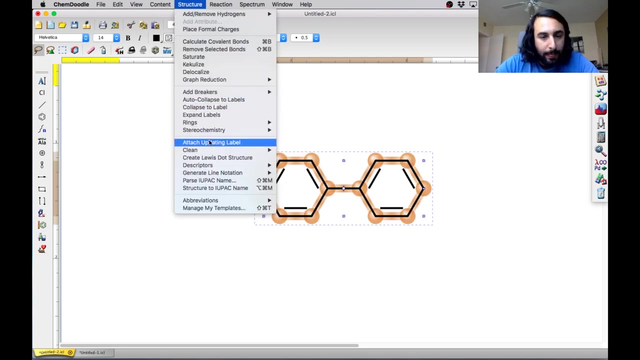 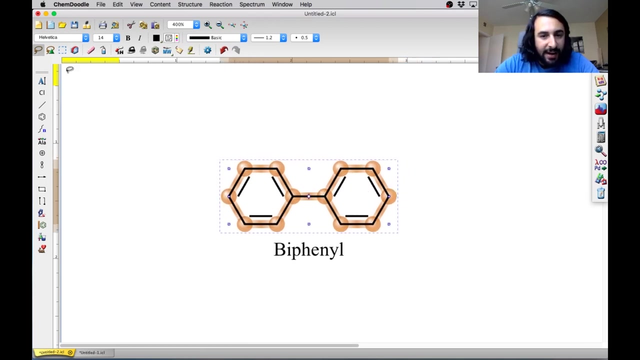 of numbers and specifically starting with the lowest number that you can. So that's naphthalene. Let's move on to another type of molecule. Let's do a biphenyl. So let's take this, Let's get the name. So there's our biphenyl. So this is different than naphthalene, right? Because 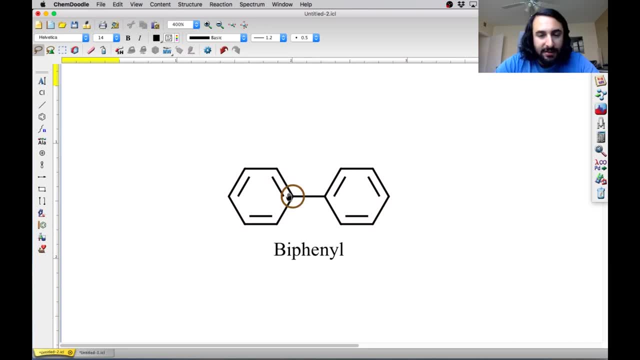 they're not fused at two carbons, We're just connected by this Single sigma bond here between these two rings. So that's biphenyl. Now let's start adding substituents. So what if we do this? So now it says orthophenyltoluene. So by adding this, 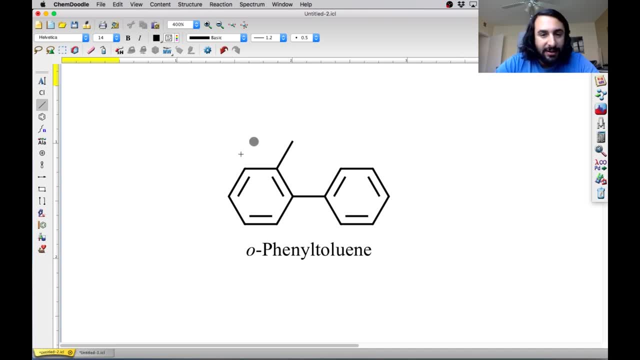 substituent. we're changing the naming scheme because we're counting this whole part as toluene right, Because toluene is a benzene ring with a methyl group on it And there's a substituent right. This is a phenyl substituent And they are specifically, they have an ortho. 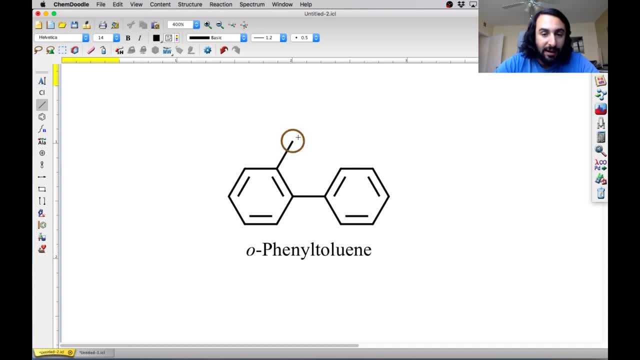 relationship to one another, because they're one apart. We have a methyl right here and we have a phenyl right here. They're one away. So that's an ortho relationship. So that's orthophenyltoluene. Now let's add another one and see what happens. So now we have 3-phenylorthozylene, So it seems. 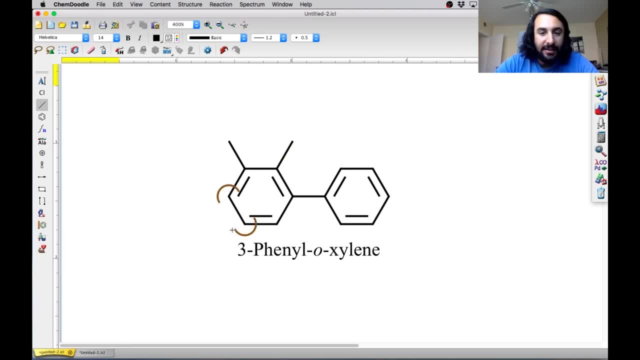 that what's happening is that we're changing the parent name on the basis of the substituted phenyl and what that becomes, Because the thing is that a benzene ring with two methyls on it is called a xylene, right? So let's, just for reference, let's show this name. 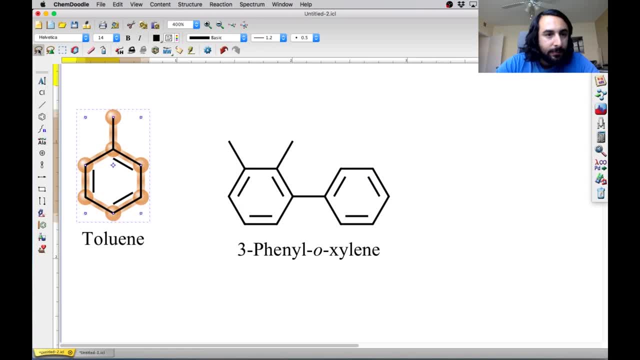 So that's toluene And we can see that that's ortho xylene And that's meta xylene And that's para xylene. So clearly, xylene is the name for a phenyl ring with a benzene ring with two methyl groups on it, And then we have ortho meta or para to describe. 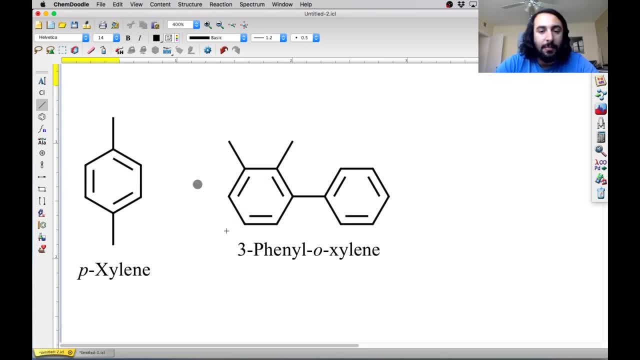 their spatial relationship. So over here we're taking this to be the main part of the molecule, We're saying that this is an ortho xylene And then, on ortho xylene, right If these are the two right carbons with the methyls there, if we go one, two, three- remember lowest number- 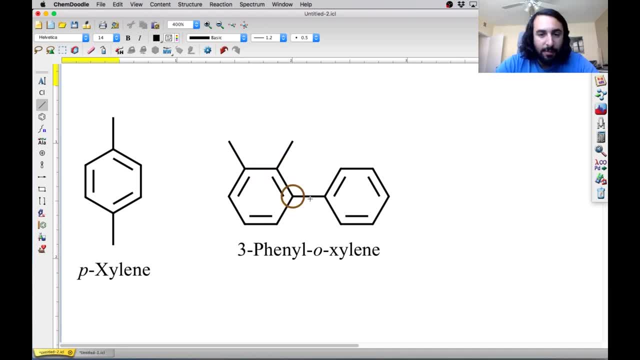 ring scheme possible. So this would be one, two, three. On carbon, three, we have a phenyl group, So that's three, phenyl ortho xylene, And we could have all kinds of fun with this. We could then come over here and start adding carbons over here and see what happens. So now three: meta toluene. 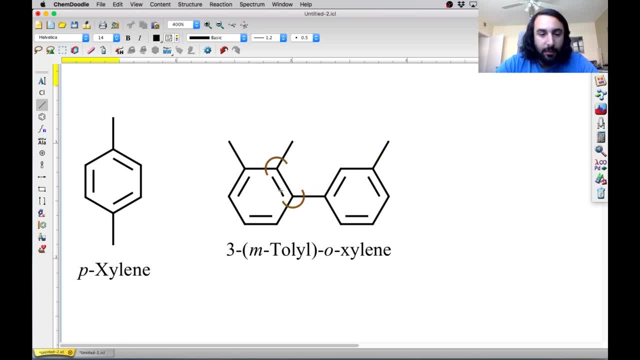 So this is now not three phenyl, but we're saying that it's a toluene because it's a toluene substituent And it's on carbon three. So this three refers to carbon one, two, three And then this meta. 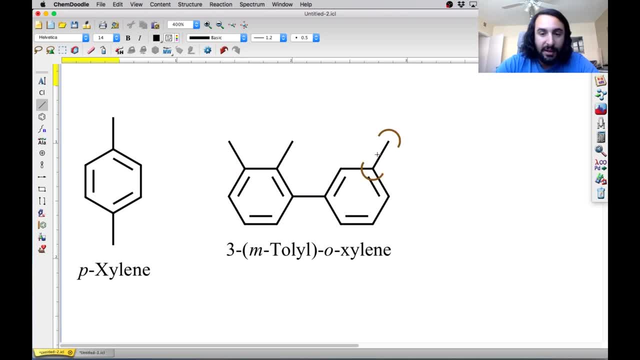 refers to this meta relationship. This methyl is meta to this whole group over here, So it starts to get pretty complicated. But what's cool about this is you can just start putting carbons up anywhere you want and see what happens to the name And, as you look at, what changes with the 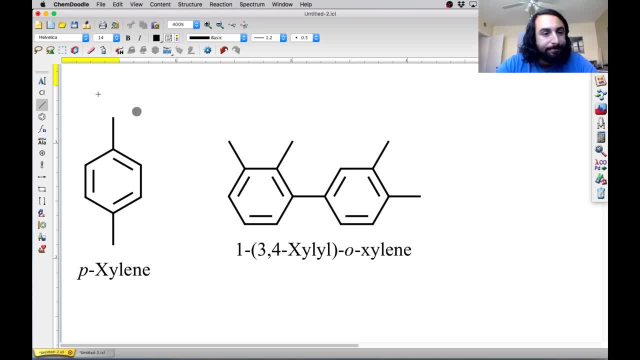 name. you sort of learn the nomenclature rules. So okay, so that's a biphenyl. Let's look at something else Now. let's look at: we did naphthalene, So let's do that was two rings put together. Now let's put three phenyl rings in this way. 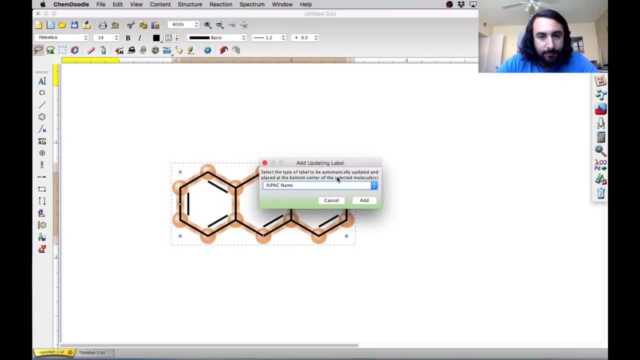 And let's get that name, And that's called anthracene. So naphthalene, two rings, three rings, we've got anthracene. And so how is this numbering scheme going to go? Let's try. let's try one there, Okay. 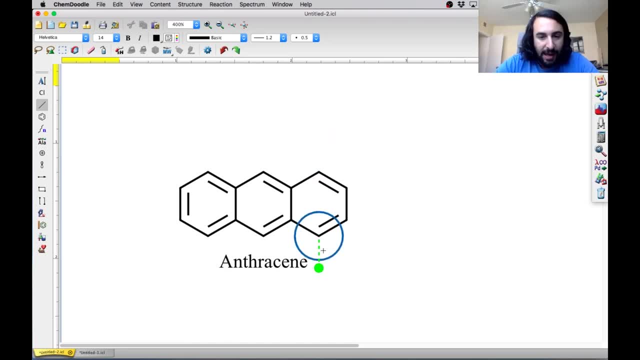 so that's one methyl anthracene. If we put that there again: one methyl, There's one methyl, There's one methyl. Okay, so clearly we've got four options here for where number one it's going to go, And that makes sense, Because if we take that molecule and we rotate it, 180. 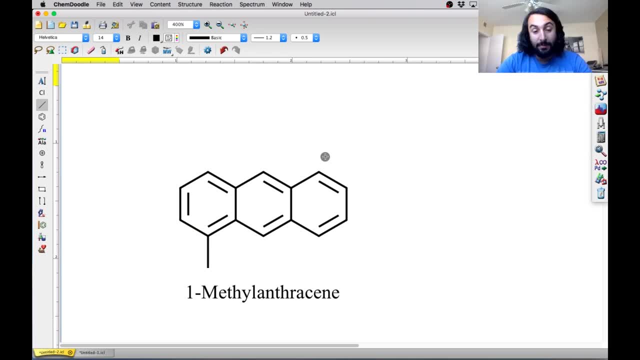 degrees like that in the plane, it would end up over here, So they'd better be the same spot. That makes perfect sense. So let's do number one. Okay, so which? which way are we going to go? Let's see what this position 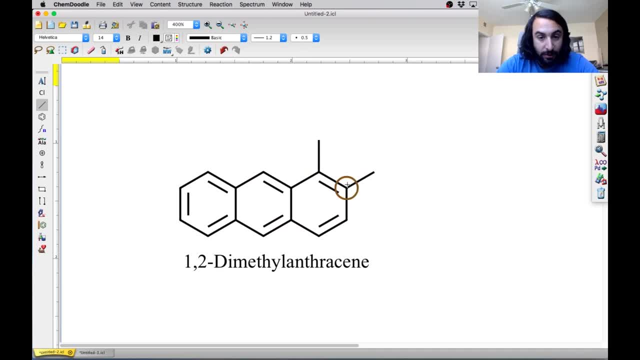 is. So that's clearly two. So we have one and two, because if we have one, two dimethyl, that's what it would be. Over there, we've got three. Over there, we've got four. Okay, so clearly we're going around the ring in this way. So 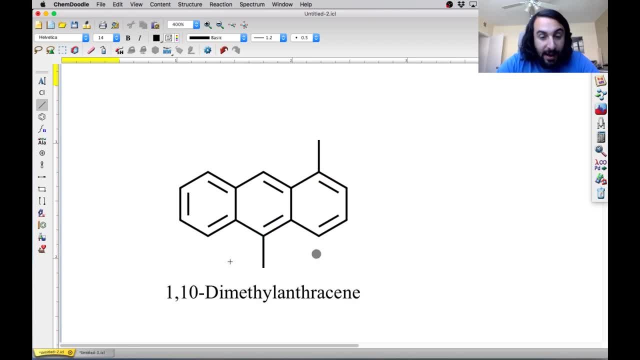 should this be five? Let's see if this is five. Now it's not, that's 10.. So what? what is five instead If we go over here? okay, so if we continue in clockwise fashion to the other edge, most ring, outermost ring. now we've. 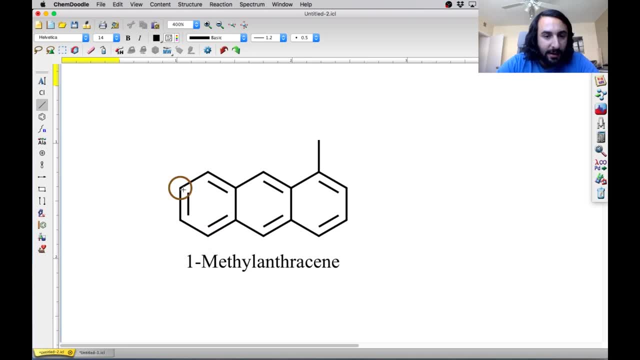 got five Now we've got six over there, Now we've got seven over there And we've got eight over there, And then we go to the central carbons, If we continue in clockwise fashion. we've got nine right there And we've got 10 right there. So we have just sort of discovered the numbering scheme. 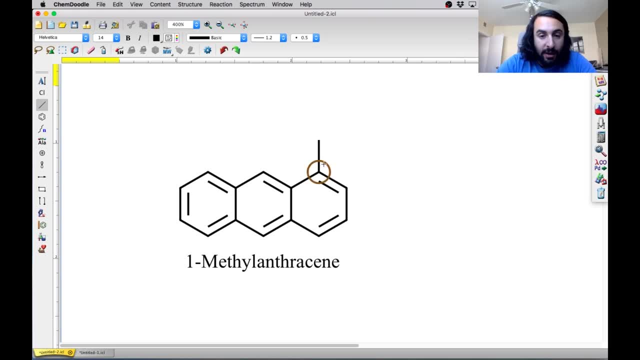 for anthracene. So we know that we're going to define carbon one, And then we're going to go around that ring. Whoops, we're going to go around that outermost ring And then we're going to skip over to the. 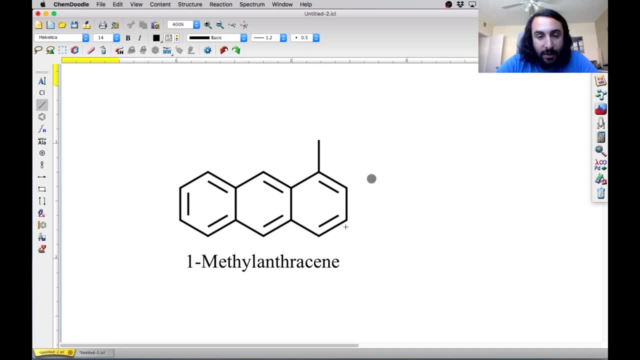 other outermost ring and finish that off before we do the middle two. So we can, we can throw some methyls on there. So this: if we put that there, we're defining this to be carbon one, because that would make this two and that's the lowest that can be. And then let's put that over here. 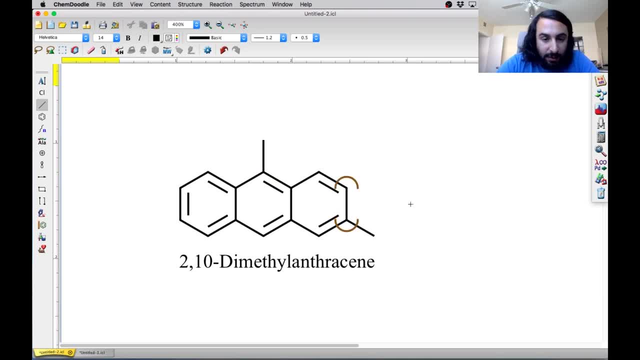 So that'd be 210.. So that's how we're going to number that, And we can just arbitrarily put a few on here and see what we get- 279.. And we can just do examples all day and see what happens to the, to the name there. Okay so, 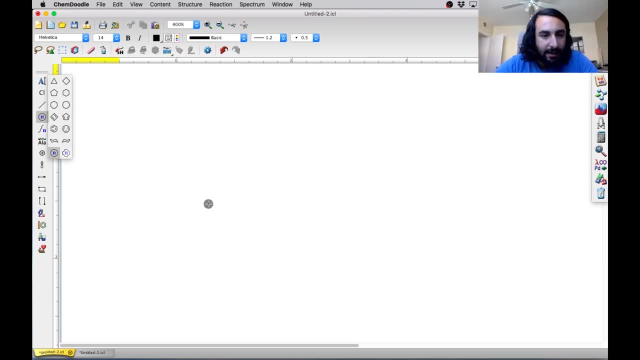 we've done some aromatic ones, Let's try some aliphatic ones. Let's try this, Let's try. We're going to take a three membered ring here, And now let's attach a ring there. Actually, before I do that, let's name it. 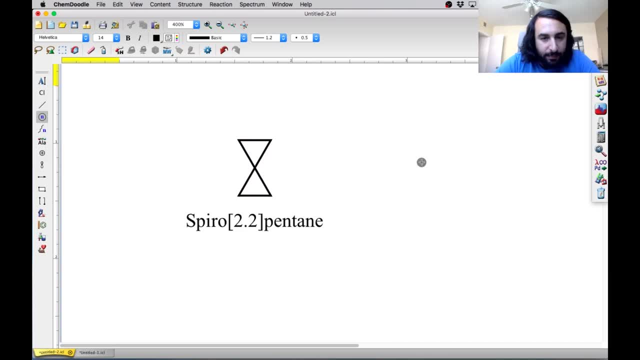 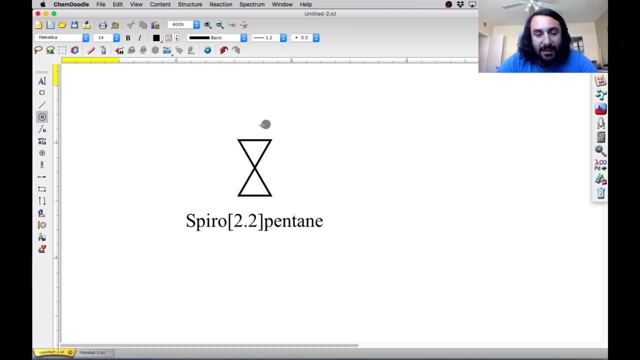 need a sigma bond between them. So that's not the, that's not the way we can go with this. Instead, we have to recognize that this is a. this is a. we're going to call it a pentane because it has five carbons, So one, two, three, four, five, but it's a Spyro compound, And what these numbers mean. 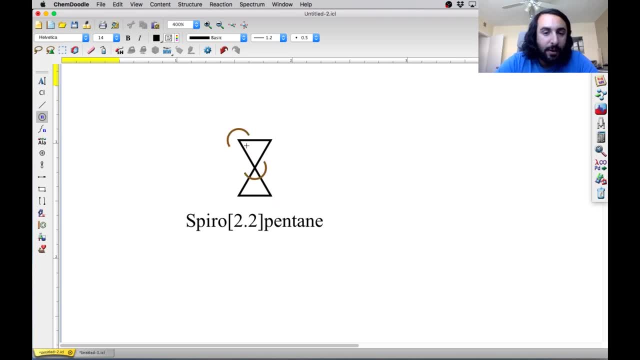 is, we're naming the number of carbons present in each ring, the one that joins them. So here's two, And here's two, And there's five total. So we say it's Spyro. Spyro refers to this orientation, And then there's two carbons here, two carbons there. 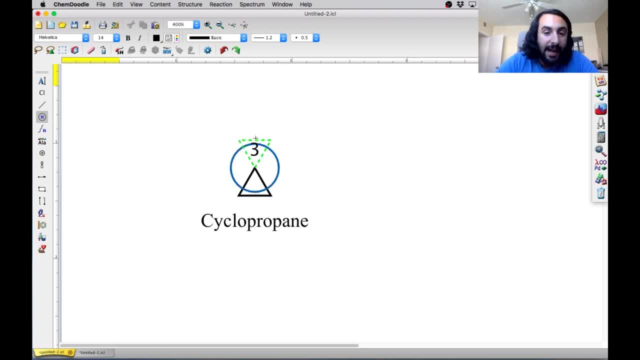 and there's five total. So it's a pentane. So what if we add a four member or a five membered ring right there? So again, Spyro, we're going to see Spyro with all of these, And then, now that we 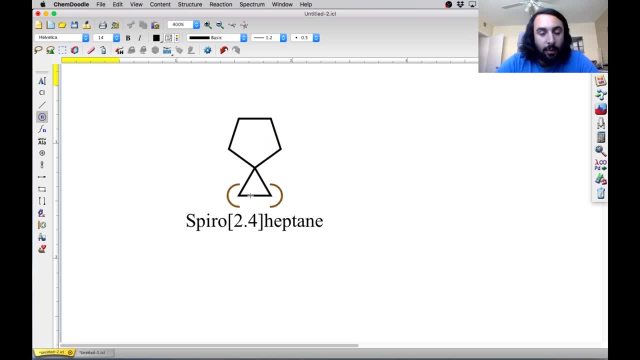 have two different sized rings. we're going to name, we're going to, we're going to refer to the smaller one first. So here are two carbons, That's the two right there, And then here's one, two, three, four. So there's four carbons there, And so four plus two plus the one that joins them. 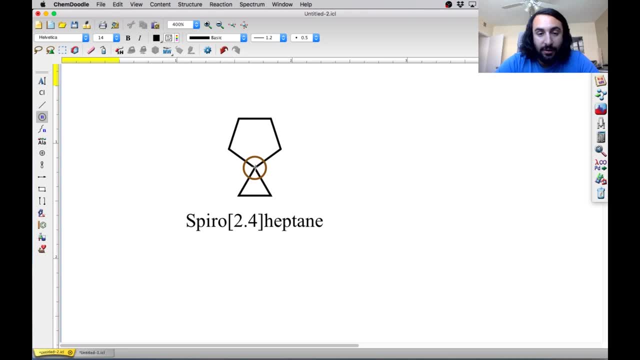 Remember, there's always going to be one more, because we're not considering this one that connects the two rings in this scheme. So add one to get seven. That's a heptane. Likewise let's put six. So again, it's pretty easy to see. It's pretty easy to see. 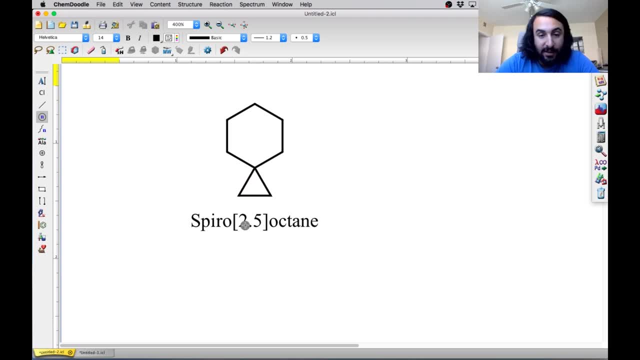 We've got a three membered ring. We don't count that one, So we've got two. We've got a six membered ring. We don't count that one, So we've got five. But then all together the five plus. 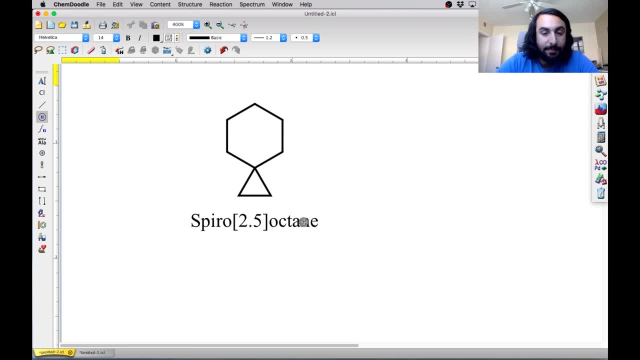 the two plus the one that joins them, That's eight. So this is Spyro two, five octane. If we want to start adding substituents, let's say like that: This is how we're going to number it. We've got. 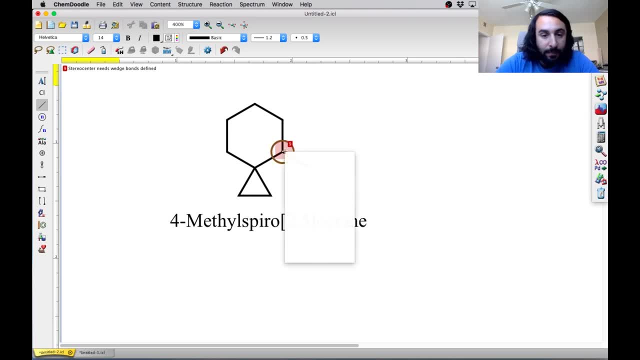 to it's. everything is the same. But if we've added a methyl group, let's get rid of that. We're going to. we're going to number from the smaller ring. So we've got two carbons here, This would be number three and then four. So that's how we're going to number. We're not going to. 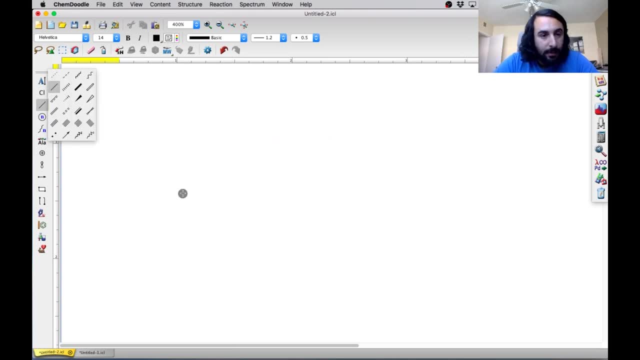 start numbering on the larger ring. We're going to start numbering from the smaller ring. OK, let's do one more type of what? one more type of compound here. Let's take a, let's do a seven membered ring And then, oh, let's get the name. So we have it. 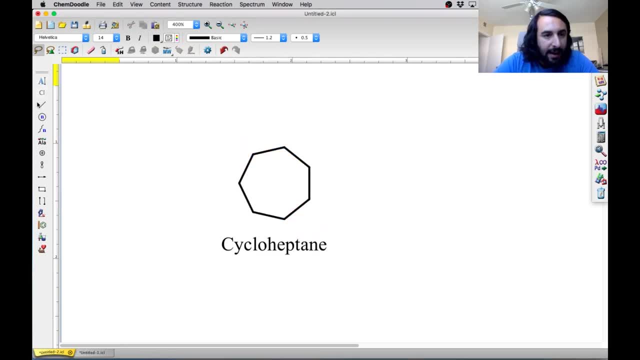 So we've got cycloheptane, And now let's make a bridgehead carbon. OK, so we've made a bicyclo structure. So the other one was Spyro. Now we're looking at bicyclo And the way that we're 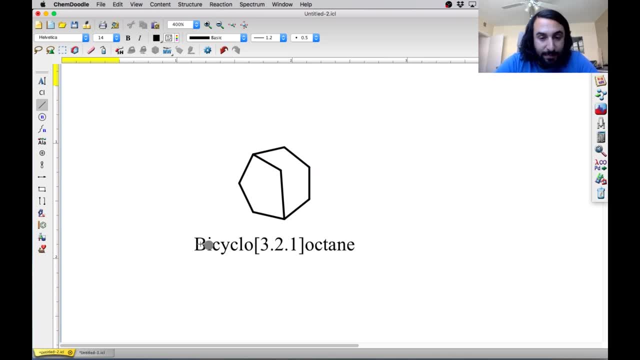 going to name these is first we say it's bicyclo, And then we're going to, we're going to just it's kind of like the Spyro, We're going to, we're going to give the numbers of carbons associated with the associated with each ring, And so we're going to go from biggest to smallest. So over here we have. 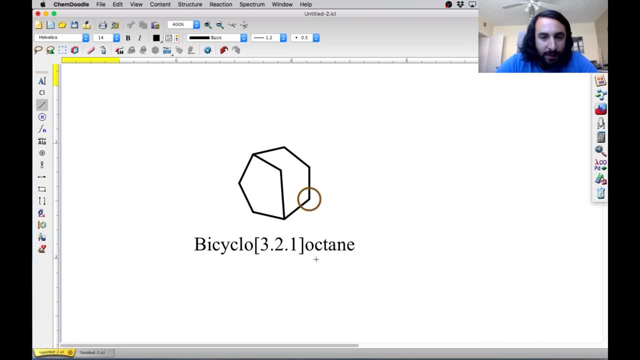 one, two, three. So that's your three: One, two, three, And then over here we have two, And so that's the two, And then, right there, we've got one. So there's your one, And total, there are eight. 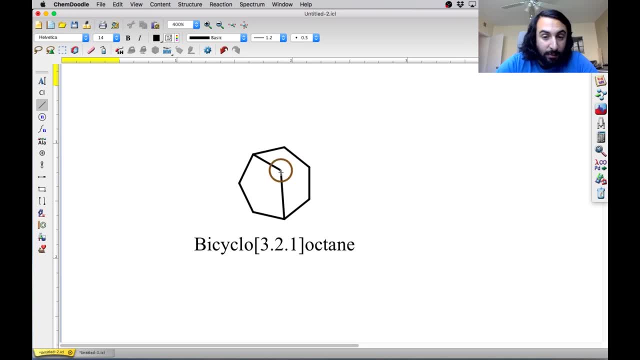 carbons. Remember we had cycloheptane and then we added one more, So that's eight, That's octane. So this is bicyclo three to one octane. Now let's do something kind of cool, because this looks. 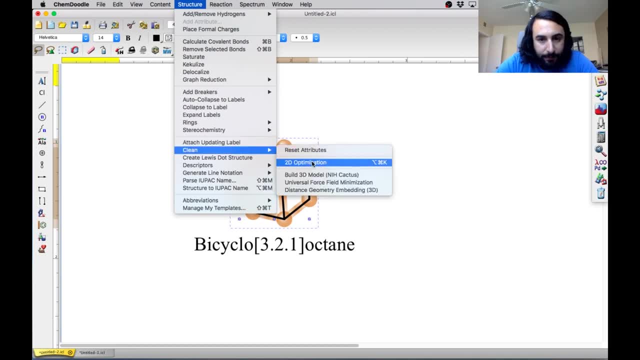 confusing. What if we're going to do this, So we're going to do this, So we're going to do this? What if we clean it up and do that? Okay, so that gives you a little bit of a better sense of. 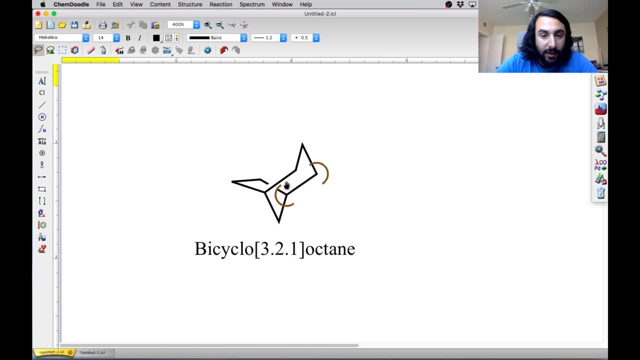 what this molecule actually looks like. We can see how you can. there's a five membered ring over here. This is a six membered ring. This is a seven. Right, If you can just kind of see the different rings in this pseudo three dimensional way, Let's do nine, Why not? 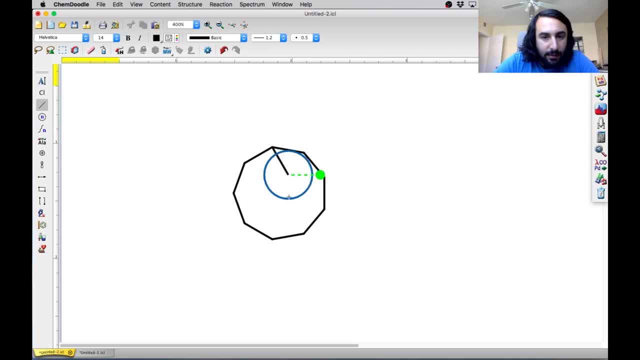 Okay, and then let's do, let's go like that. So what do you think this is going to be? It's going to be bicyclo. And then how are we going to number this? Remember, we've got the most first, So one, two, three, four- we need the four- And then we've got three, And then we've got.